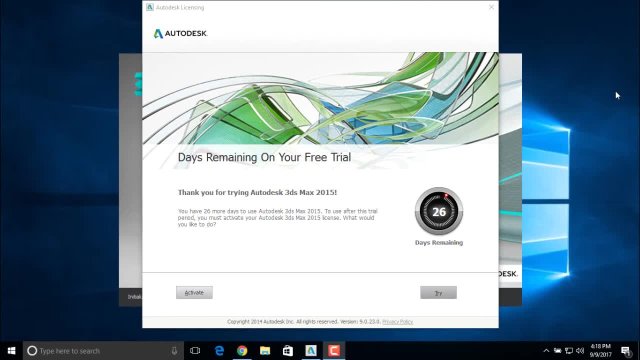 like a Maya or Max, you need to have a 3D software. If you want to use a Autotext software like a Maya, purchase it or you can also try it for 30 days. So here you can see. I download Autodesk Maya from the website and use it for the 30 days. This is the screen of 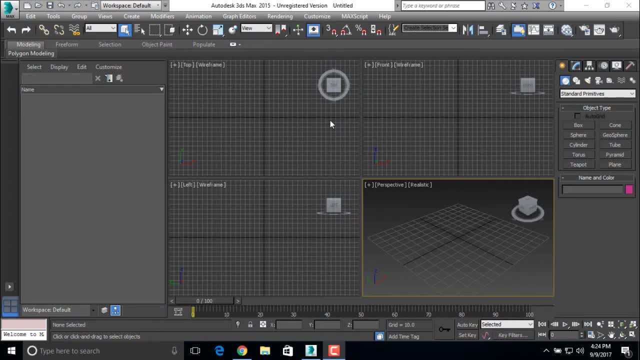 Autodesk 3DX Max 2015.. Here you can see a different view called a top view, left view, front view and perspective view. Now create any 3D model. you need to know a basics parameters. Here you can see a edit tools groups view. create modifiers. 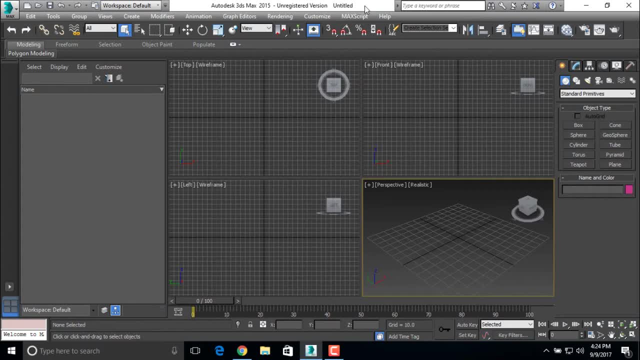 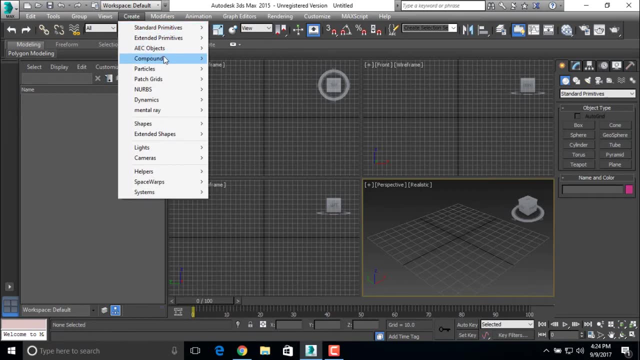 animations and many more. option For create a 3D model. you need to go for a create. Here you can see many options. If you want to create a simple object, you can use a standard primitive. You can also see these over here: Standard. 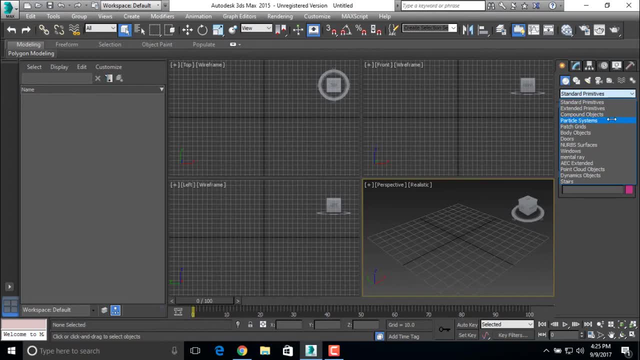 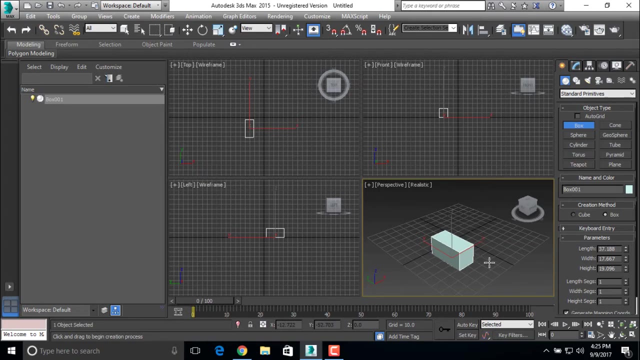 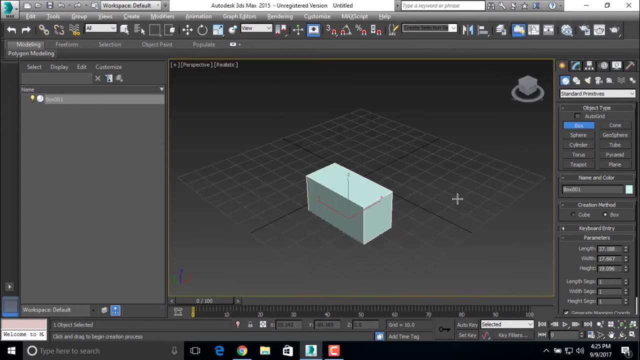 primitive, extended, primitive, compound, primitive objects, particle system and much more. So now we are going to create some 3D object. Okay, but I have to maximize this view For that place. control plus W, So you can do your work easily If you press Alt and a scroll click so you can toggle. 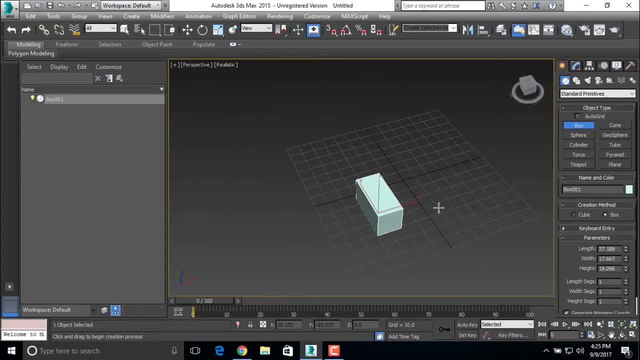 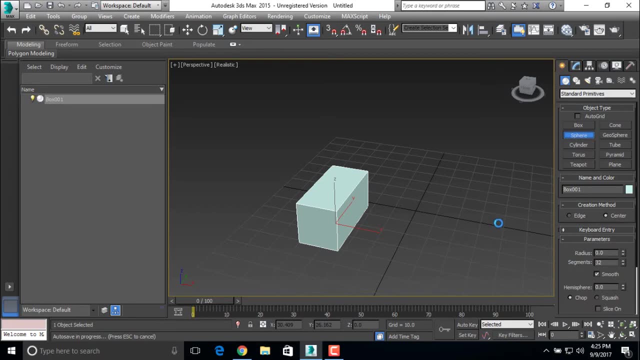 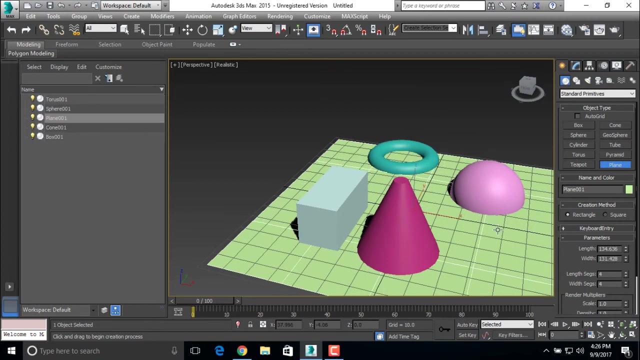 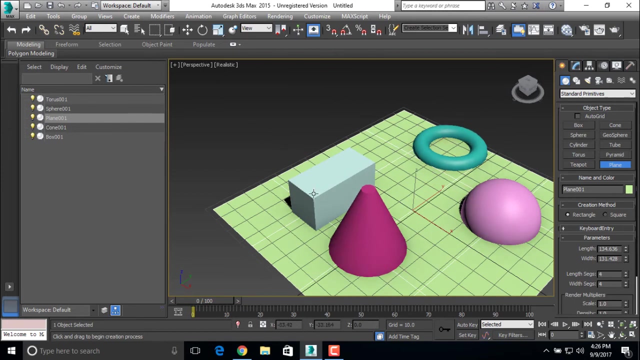 your view And scroll in, scroll out to zoom in and zoom out your view. So I create a box, can do a modification in that model and this is a plane. so in a 3d you can create a different kind of model. now if I want to move this model I click on the move button so I can select any model and 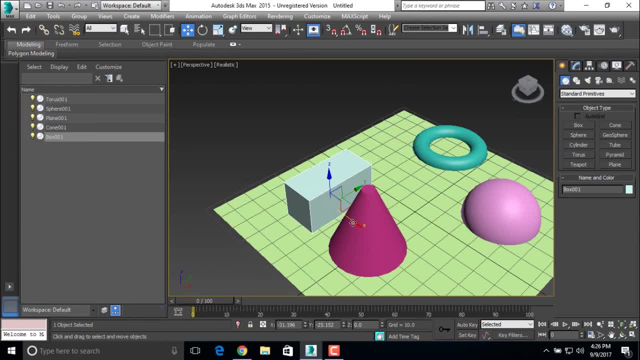 move it on Y direction, X directions or even a Z direction. so this is a simple example of how you can create a simple modeling in 3d max.